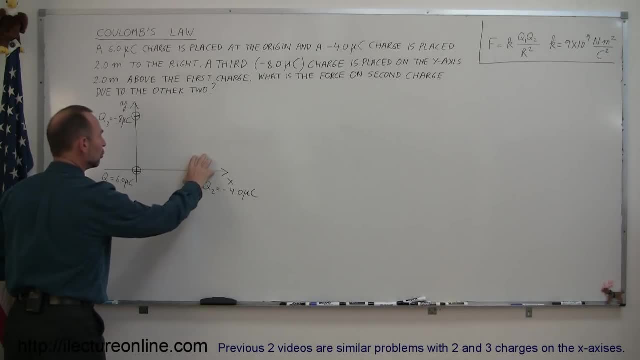 vectors representing the forces on Q2 due to the presence of these other two charges. So, for the presence of Q1, what happens to Q2?? Well, since they're oppositely charged, Q2 is attracted to Q1, so there's a force in this direction. 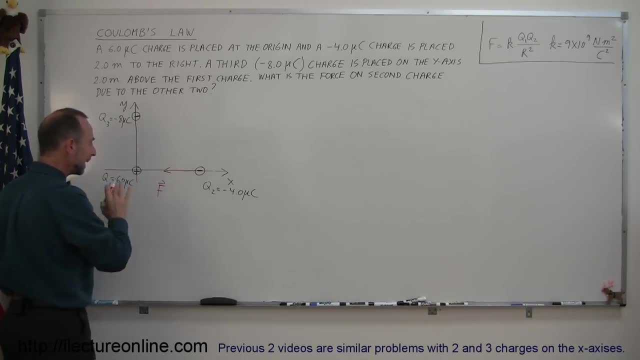 and let's call that F, and to indicate that this is the force between Q1 and Q2. what I do is I go F1, comma 2.. So I know it's a force between these two and it's in the left direction. OK, so now we have another charge, and so how does this charge affect this charge? 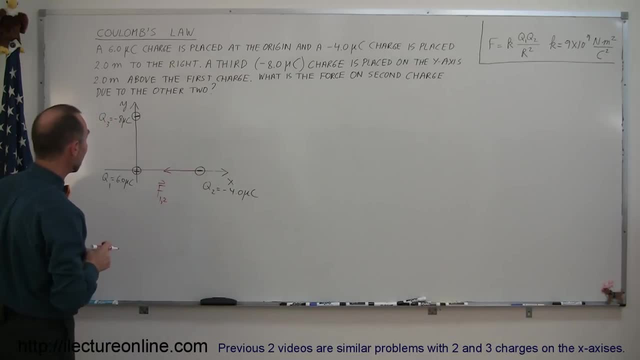 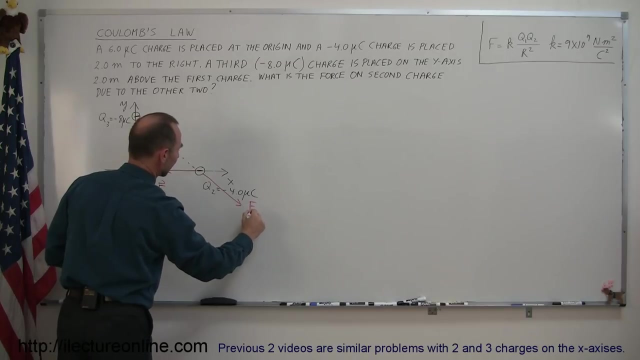 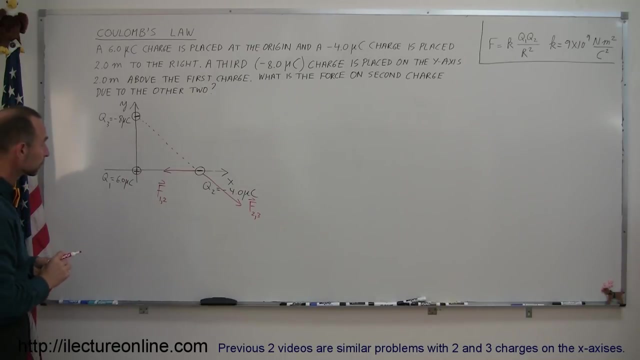 Now, since they're both negatively charged, they repel each other, and so that means that this charge pushes against this charge in this direction, And so we have a second force in this direction. call that F between 2 and 3, and that gives you kind of a visual explanation as to those forces. what 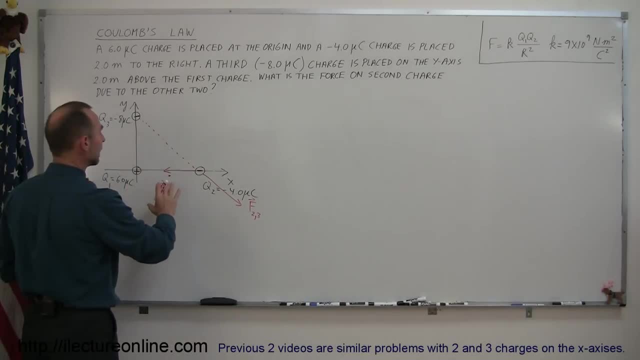 those forces are. Now, what it ends up being is simply a vector sum of these two forces to find out what the net resultant force is. And before you get started on that, you may want to say, well, let's see, I want to have kind of a 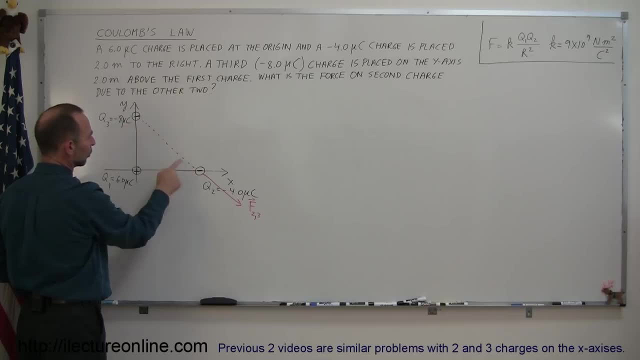 visual picture of how big these forces are. This is an eight microcoulomb force and a four microcoulomb force. They're both negative and so they're about this far apart. and this is six and four, and they're a little bit closer together. so 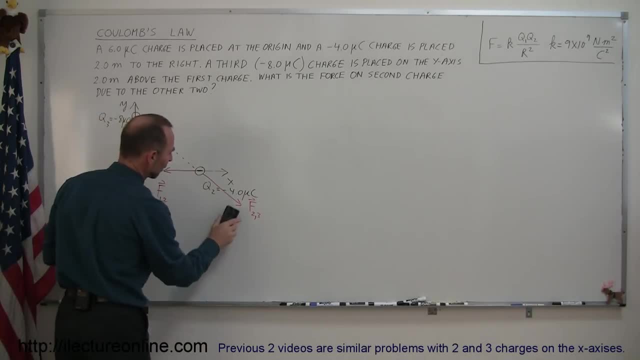 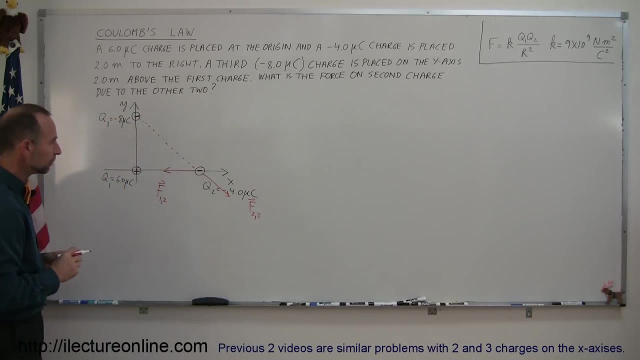 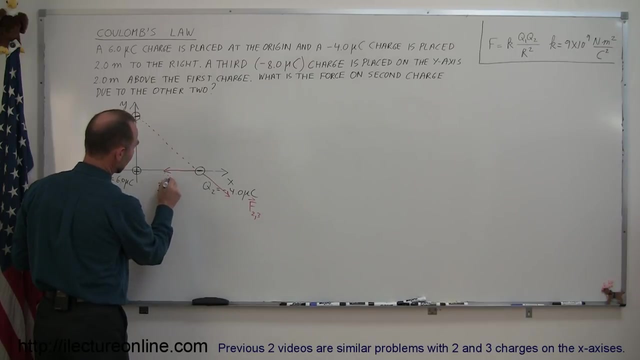 it looks like the magnitude force is probably about the same. So I want to give it a fairly good visual picture that is reasonably correct on the magnitude of those two forces. So I can graphically now say well, the sum of these two forces graphically, using what we know as a parallel government method. 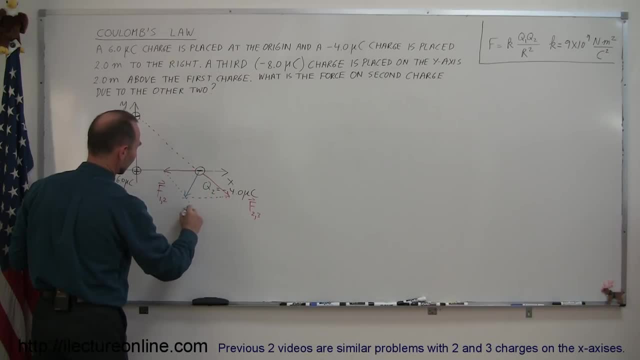 you can then see that the net force or total force, F, total- would be kind of like this: So that's what we're looking for. that's the answer, and, of course, to find the answer, we didn't have to find the magnitude of that force and the 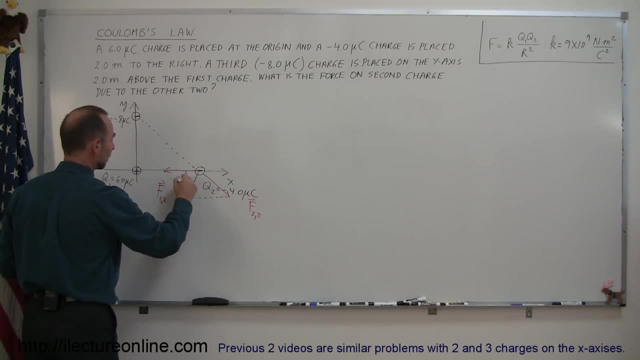 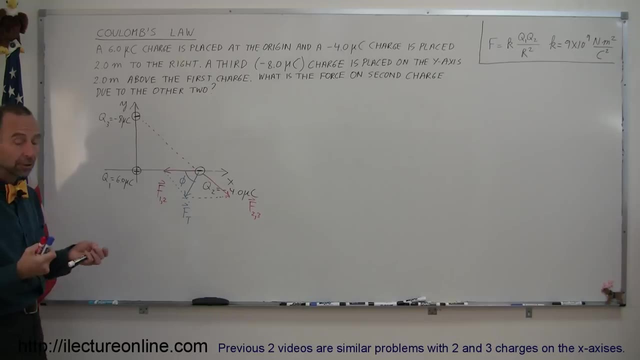 direction of the force. For example, we want to find the angle- let's call it phi- between that force and the, the x-axis in that direction. Alright, so how do you go about doing that? Well, the first thing you want to do is actually find the magnitude of these two forces. So, using Coulomb's law, we 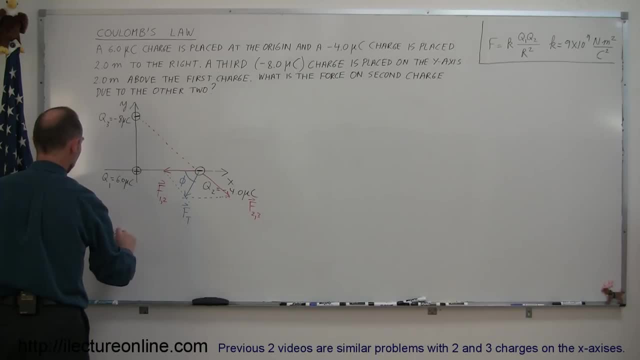 can say that F1, 2 is equal to. and I'm going to write it like this to indicate again that I'm finding the magnitude of that force, not the magnitude and direction, simply the magnitude. it's a scalar quantity. It's kind of like the. 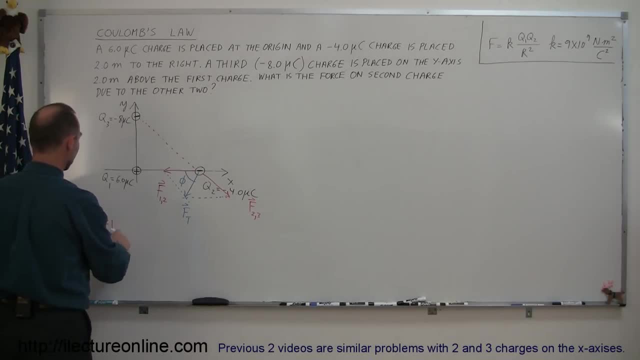 absolute value of that result, and it always will be positive. and so this is equal to k times Q 1, Q 2 divided by the distance between one and two squared. Now again, I use this subscript 1 and 2 to indicate that I'm looking for the distance. 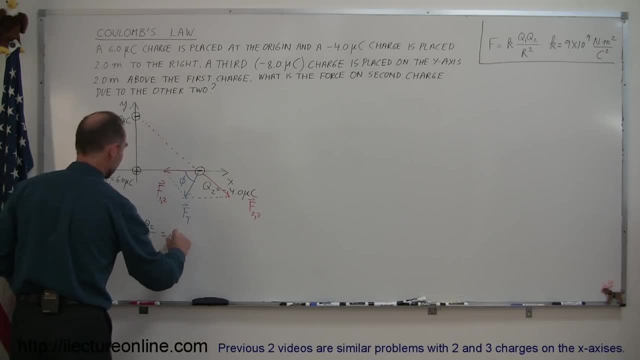 between those two, And this is equal to 9 times 10. to the 9th newtons, meters squared per kilogram squared. Well, not kilogram squared, I keep thinking about Newton's law, but no, Here we're dealing with charges, so it's coulombs squared. Multiply the times, the magnitude of the first. 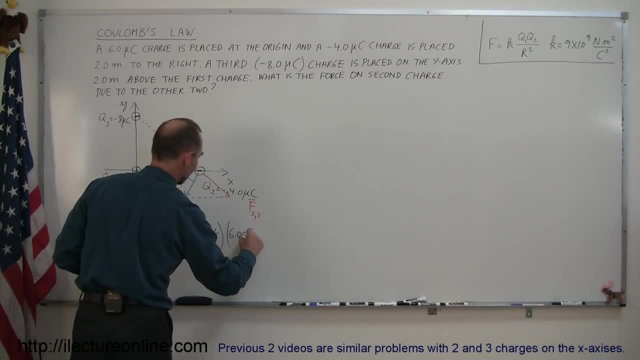 charge, That's this one right here. So it's 6.0 times 10 to the minus 6 coulombs, because micro is 10 to the minus 6.. The second charge is 4.0 times 10 to the minus 6 coulombs Again, even though. 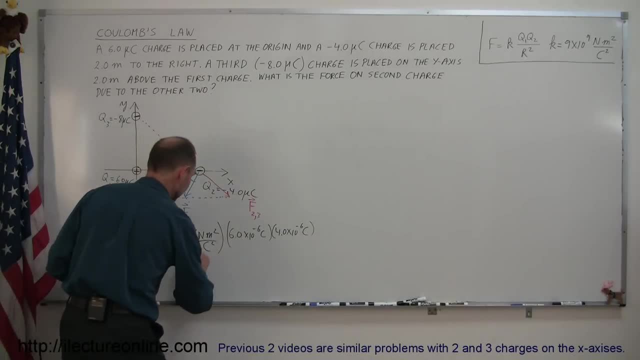 it's negative. I put a positive quantity in, because that is just the magnitude that we're looking for, And then the distance between them squared, we realize that this distance here is 2 meters, So we write 2.0 meters coulombs. 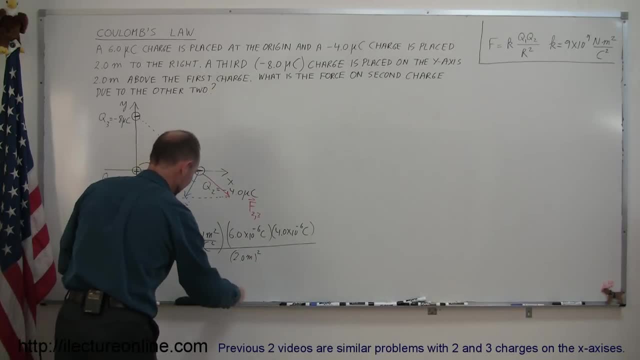 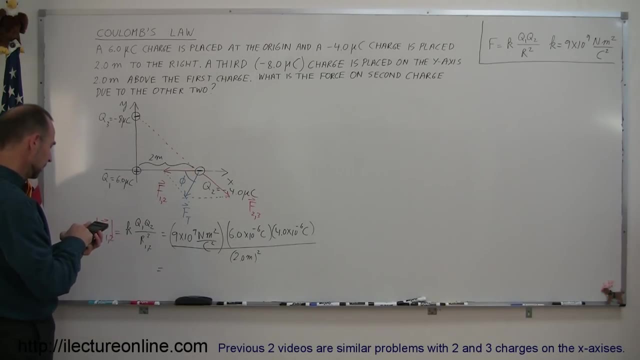 Quantity squared, And then we grab our calculator to find out what the magnitude of that force is. So plug in numbers. So it's 9e to the 9th times 6. exponent to the 6 minus times 4e to the 6 minus. 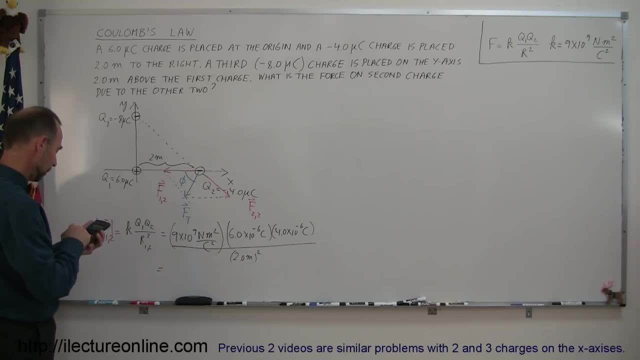 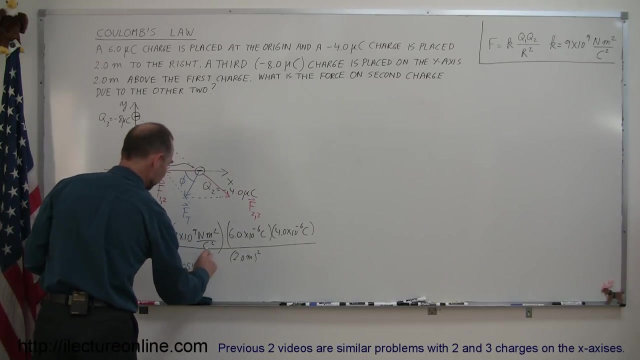 equals, And then we divide that by 2 squared, So that's 4.. And the answer? where did my pen go? The answer then becomes 0.054, and that would be newtons. The force is in newtons. Notice that the coulombs squared. 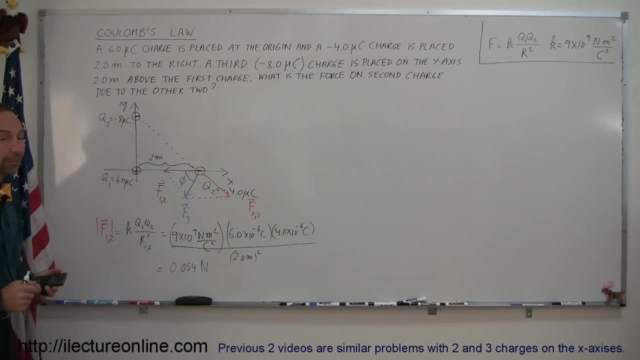 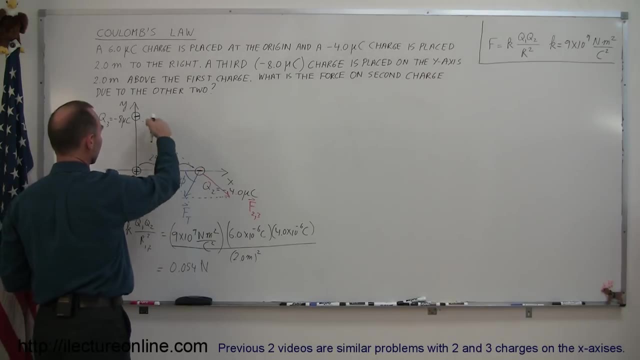 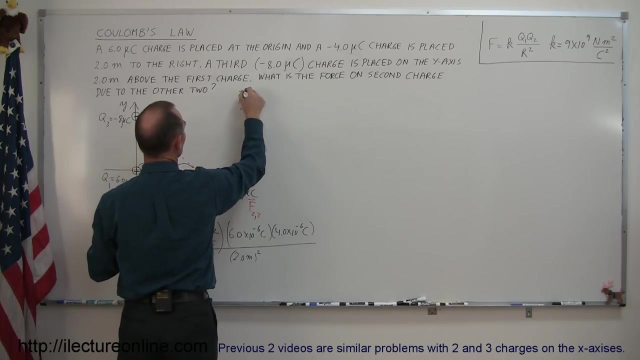 cancel out and the meters, squared, cancel out, So we're left with newtons. So that's the magnitude of the force between those 2 charges. We do the same for the other 2 charges. We now want to find the magnitude of the force between those 2.. So we can say that F between 2 and 3, and again. I indicate that it's the magnitude that we're looking for And that's how we'll phrase it. And once again we do the same thing for the other 2 charges, Just the magnitude of the force between those 2.. That's the answer, you see. And once again set the magnitude between the 2 and city. Now 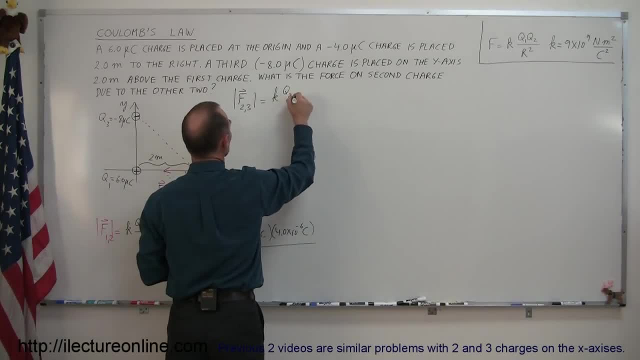 what we're looking for is fuerza between ciudad. if we see this, what we're managing is these: 2 and 3, is equal to K times Q2 times Q3 divided by the distance between them squared. So again, I will indicate that the distance between them squared is R2,3, subscript 2 and 3.. 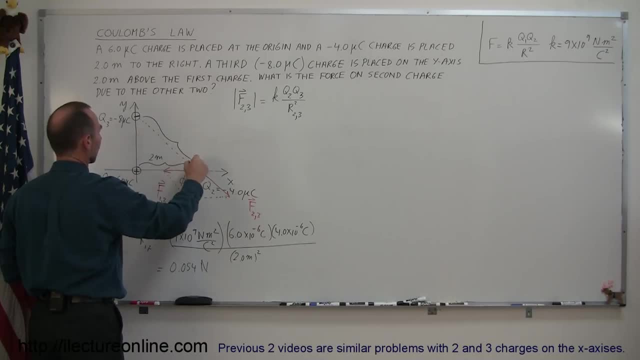 Now, what is this distance? This is R2,3.. What is this equal to? Well, since we know that this distance is 2 meters and that distance is 2 meters, and that's a hypotenuse, we can kind of use Pythagorean theorem. 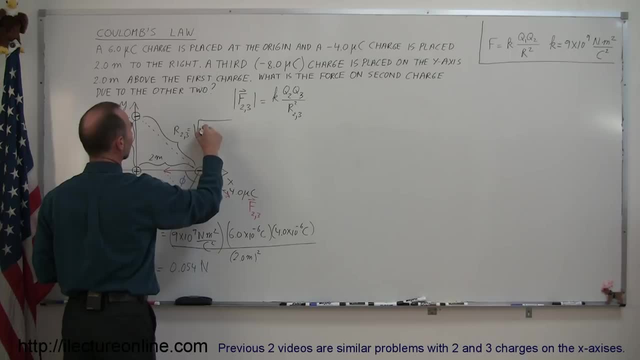 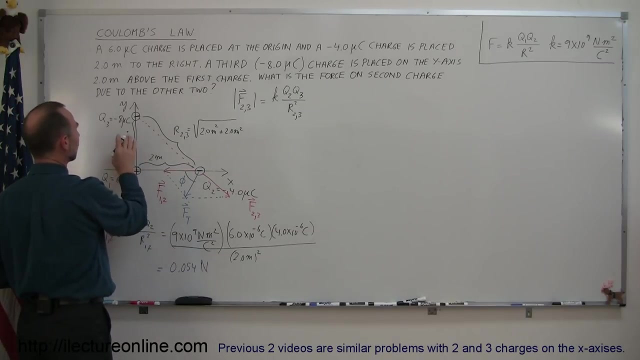 We can say that that distance is equal to the square root of 2.0 meters squared, plus 2.0 meters squared. Remember that the magnitude of a diagonal of a square or any triangle is equal to the sum of the squares of the two sides. 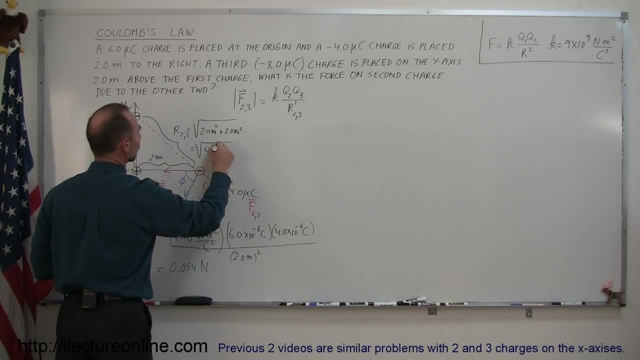 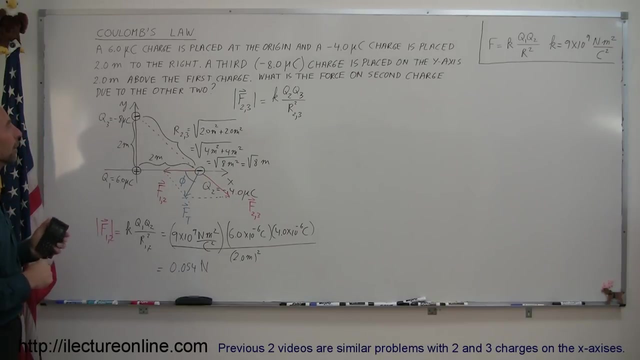 So this would be equal to the square root of 4 meters squared, plus 4 meters squared, which is equal to the square root of 8 meters squared, And so that's 2.0 meters squared, equal to the square root of 8 times meters. Alright, now plugging in the. 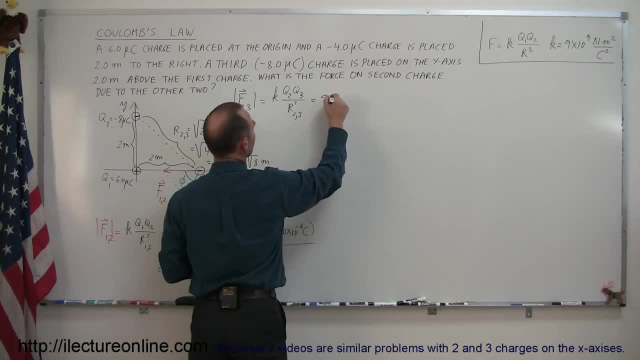 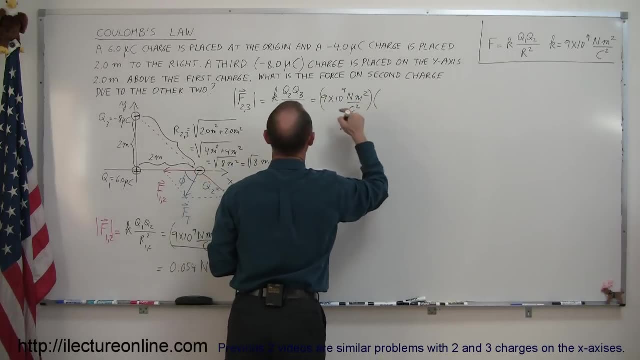 values that we have. this is equal to 9 times 10 to the 9th Newton's meters squared per coulomb, squared times the charge 2.. Charge 2: right here is again. I use the positive value times 10 to the minus 6 coulombs, then Q3, which is over. 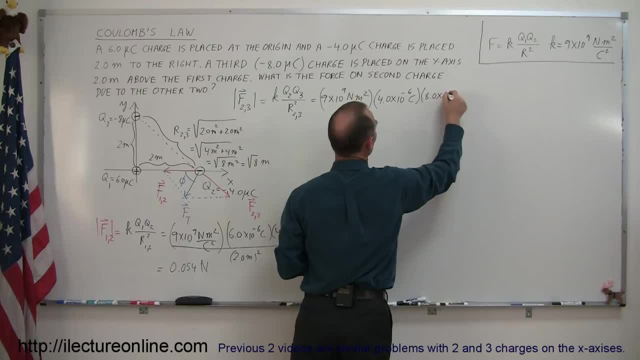 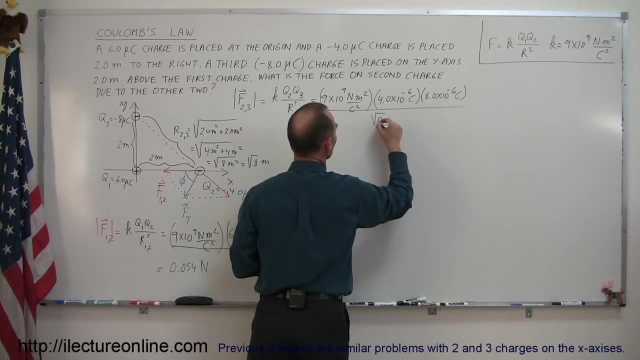 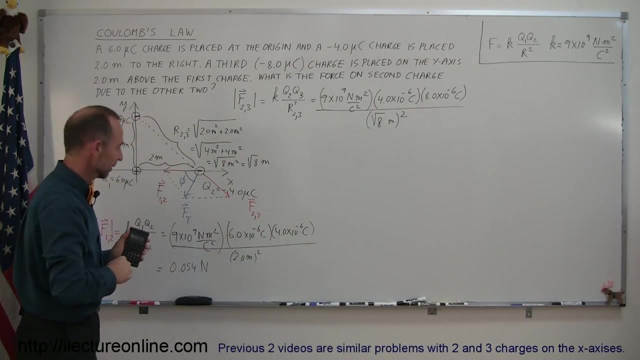 here I use 8.0 times 10 to the minus 6 coulombs and take the whole thing divided by the distance between them squared, so that would be the square root of 8 meters, quantity squared. Alright, now we can go ahead and use our trusted 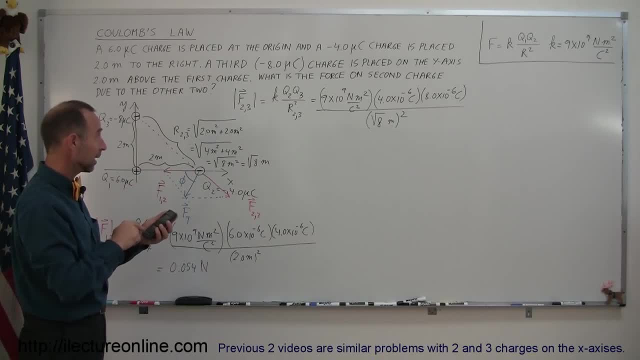 calculator to find out what that is: 9e to the 9th times 4e to the 6th minus times 8. exponent 6 minus equals and then divided by the squared of 8, squared of course, the squared of 8 is: 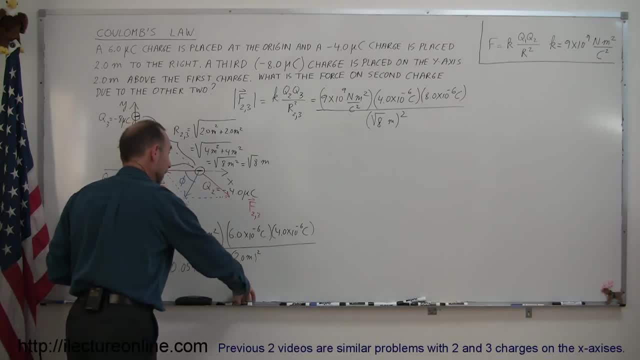 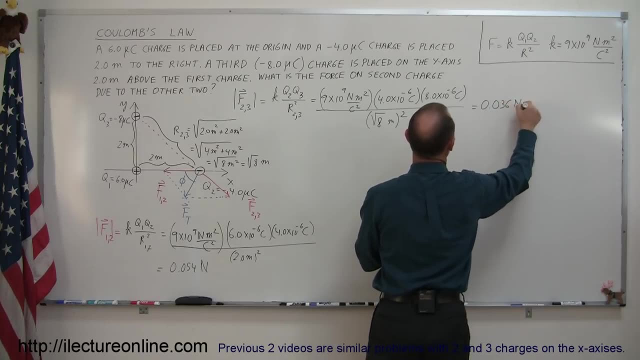 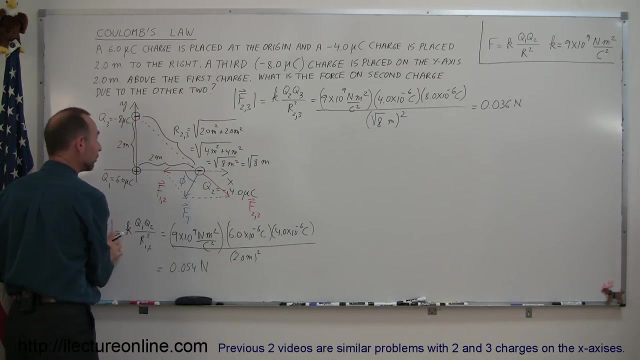 8. so divided by 8 equals and the magnitude there is equal to 0.036 Newton's. Again, the meters squared cancel out and the coulombs squared cancel out. Alright, so now we have the magnitude of f12, we have the magnitude. 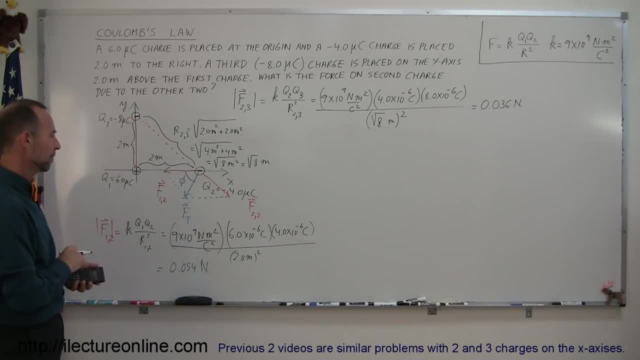 of f23.. What do we do next? Well, since we're going to have to add them as vectors, We can't just these two numbers together. they're pointing in different directions. so to solve that, we have to find the x and y components of each of those vectors. Now, 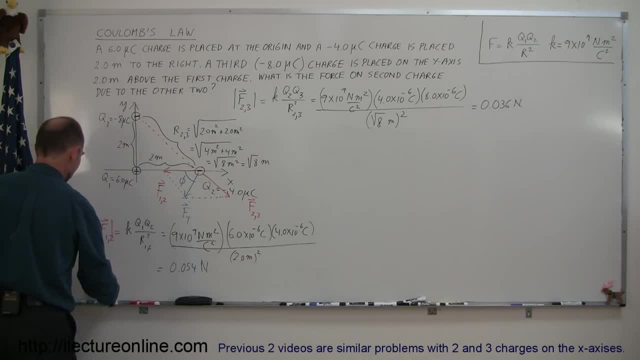 for F1,2. that's fairly easy. We can say that F1, the magnitude in the x direction, or I should say F1,2, not F1, but the force between 1 and 2, 1 and 2 in the. 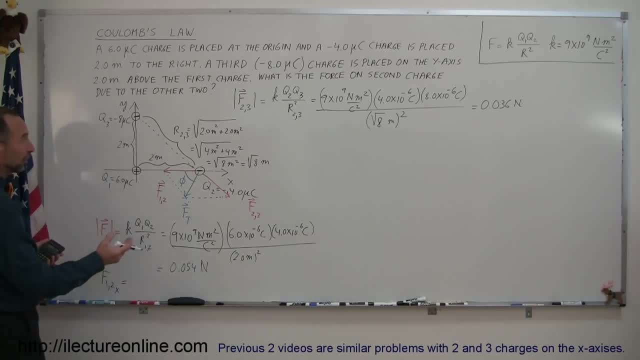 x-direction. that is simply equal to the magnitude of that, because the force is pointing in the x-direction. so the magnitude of that is equal to 0.054 Newtons. So well, wait a minute. isn't it pointing to the left, Shouldn't that be? 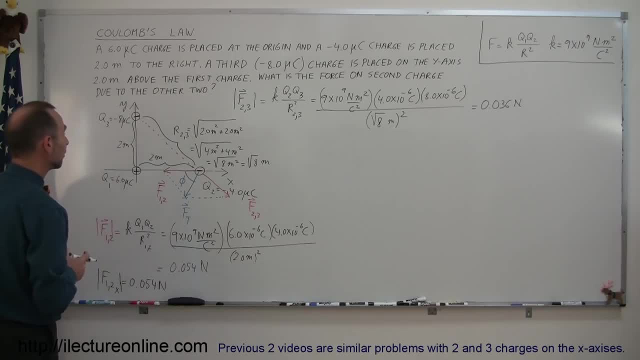 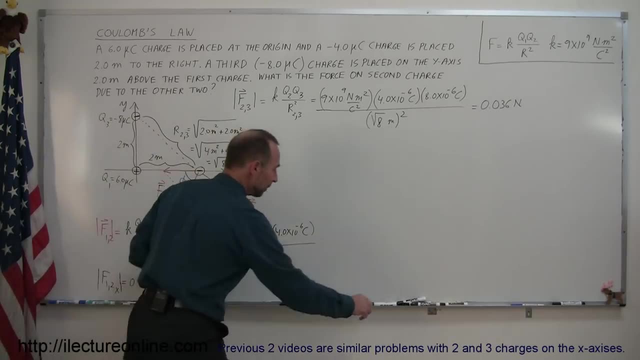 negative Again, since we're looking for the magnitude. it's just a positive quantity, It's an absolute value. Now we have to do the same for F2,3.. Now here it's a little, a little bit more tricky because we have to find the x and y. 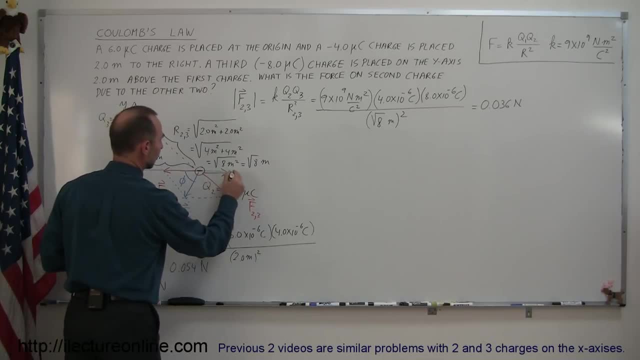 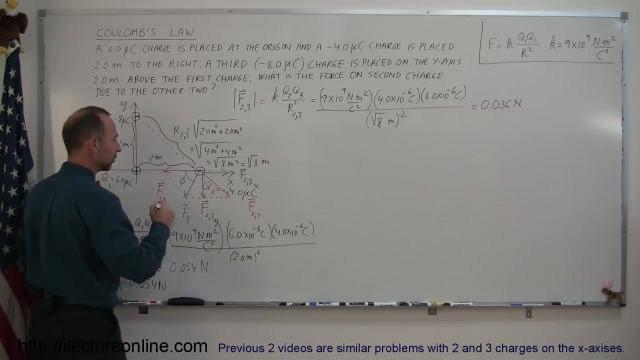 components of that force. So in other words, here this would be the F1,2,3. in the x-direction, and here this here would be the F2,3 in the y-direction. We then have to realize what this angle is, This angle, here is theta, Now here. 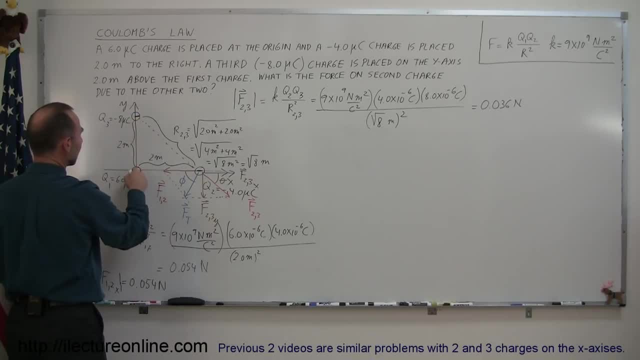 it's fairly simple on the angle, because we know that this is a side that's equal to 2 meters. this side is equal to 2 meters, so we know that this is directed 45 degrees below the horizontal. This is therefore 45 degrees, so we can say that. 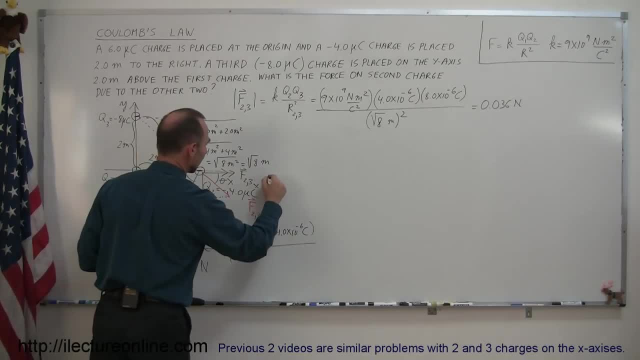 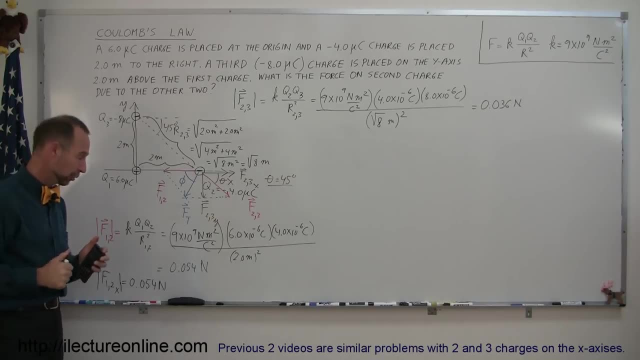 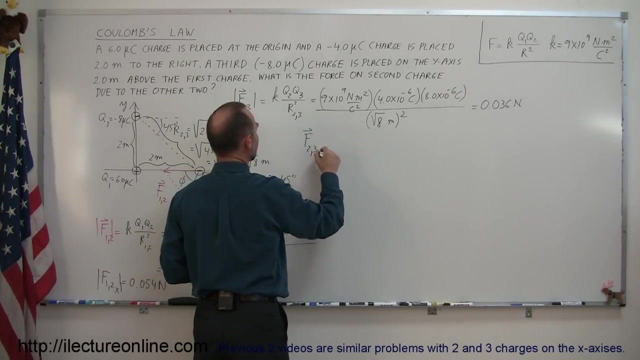 this angle here is 45 degrees, So we can say that theta is equal to 45 degrees. Alright, knowing that, let's find the x and y components of F2,3.. So F2,3 in the x-direction is equal to, and again, I'm only looking for the magnitude. so far so. 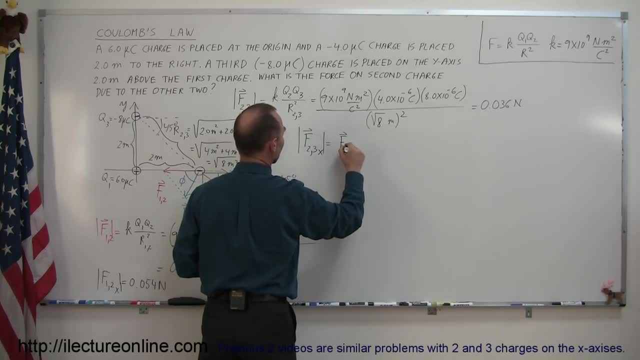 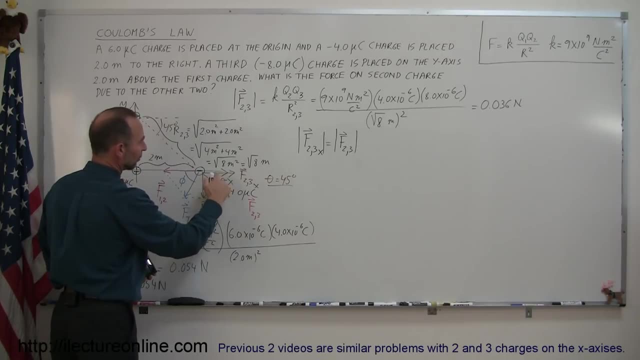 that is equal to the vector F2,3, or the magnitude of the vector times D. So if we, Since the x component is adjacent to the angle of this particular triangle, we can say that this is equal to the cosine of theta. 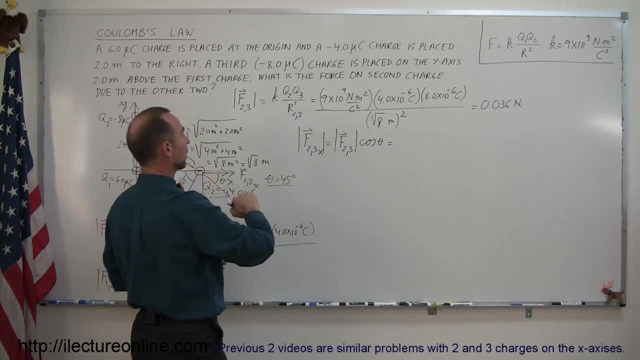 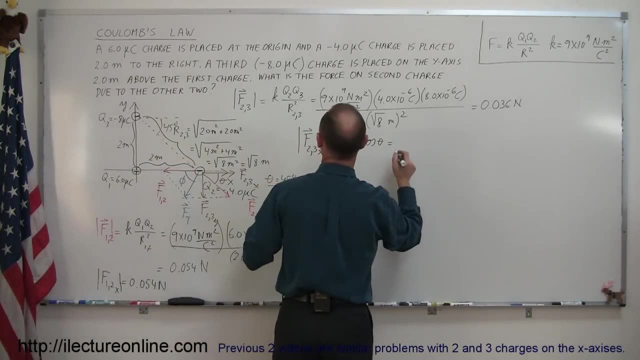 And so this is equal to the magnitude of F2,3, which is right here. It's a good thing that we label the subscripts of what these forces are, Otherwise we get confused. So make sure you use a good labeling technique. 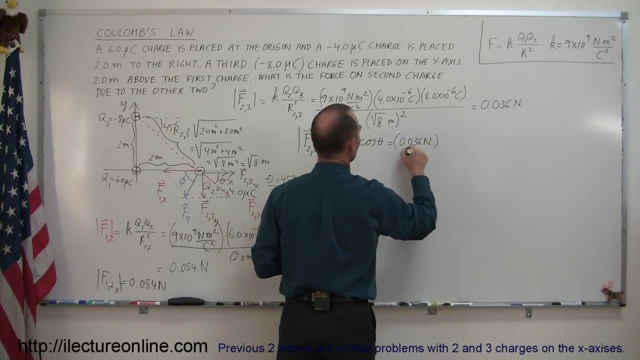 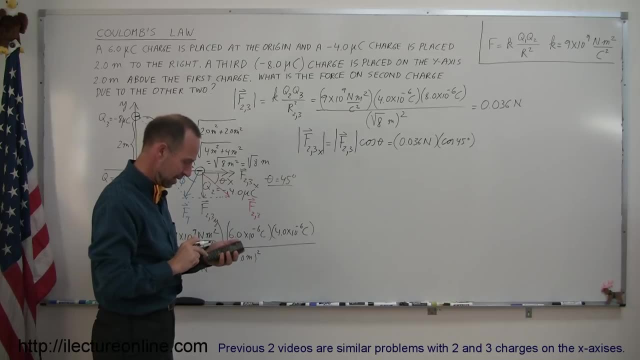 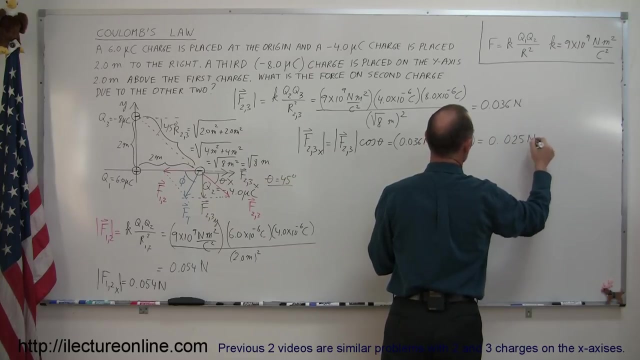 So it's 0.036 newtons times the cosine of 45 degrees, And so times 45 cosine equals, and so this becomes 0.025 newtons. So that's the x component of F2,3.. Now we do the same for the y component. 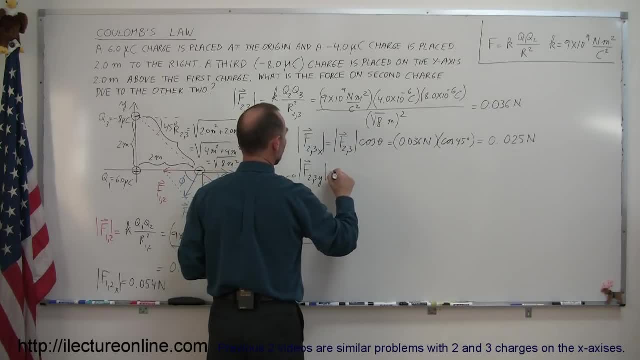 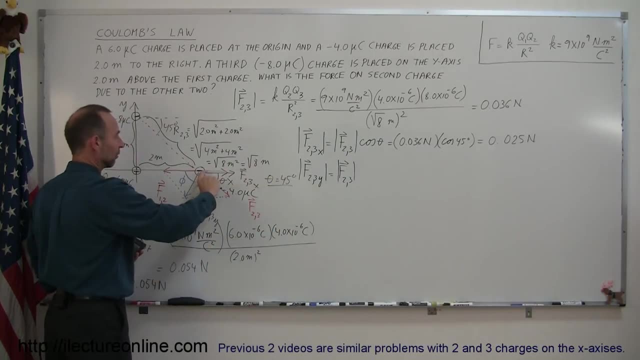 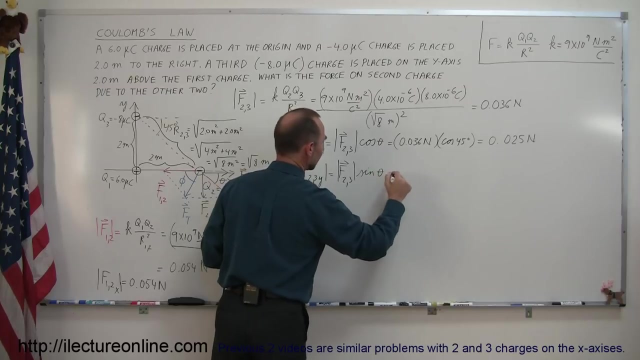 So F2,3 in the y direction is equal to F2,3 times. in this case, since we can move this vector over here, that would make it 0. If we make it opposite to the angle theta, we can say that's equal times the sine of theta. 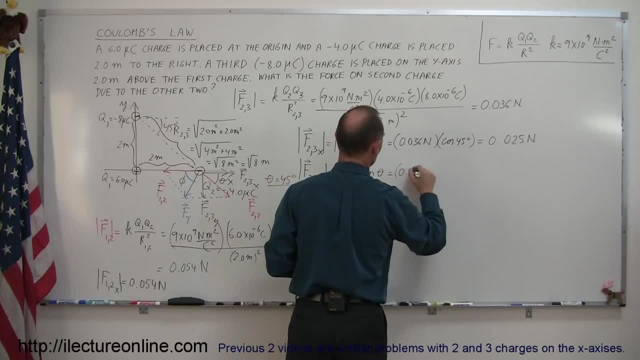 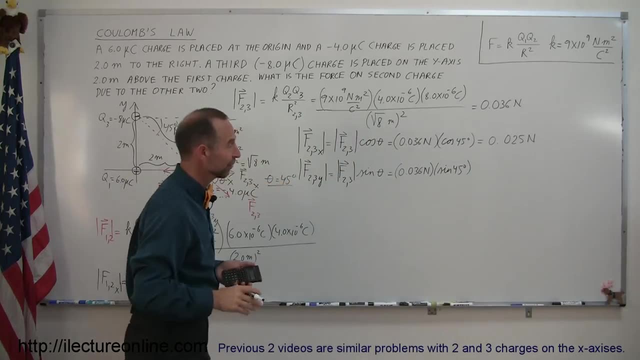 All right, plugging in the numbers here, we can say that this is 0.036 newtons times the sine of 45 degrees, And of course we should know that the cosine of 45 degrees and the sine of 45 degrees are the same. 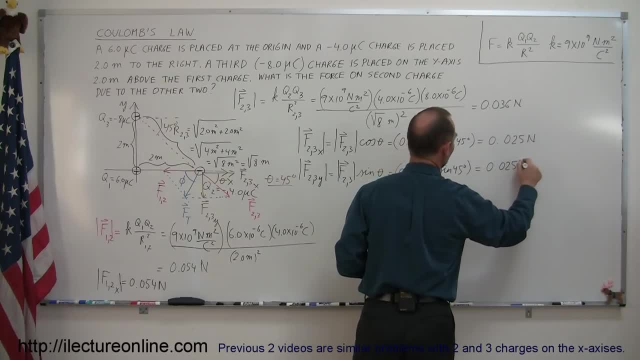 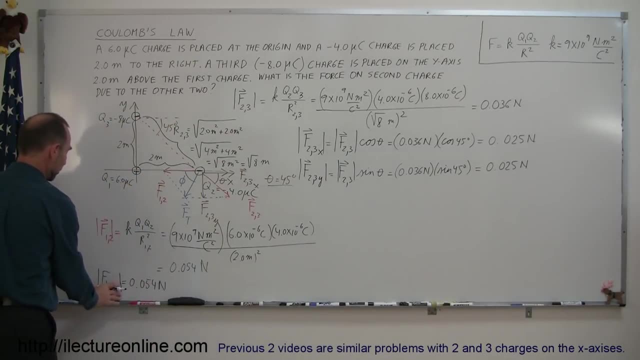 so we'll get the same answer: 0.025 newtons. Okay, now we have all the components of each of the two vectors. We have the x component of F1,2.. The y component of F1,2 is 0,, so we don't need to calculate that. 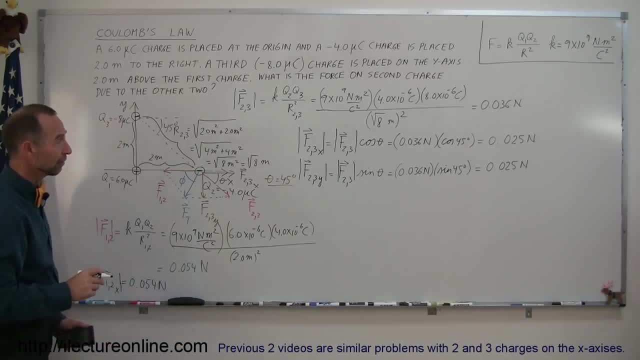 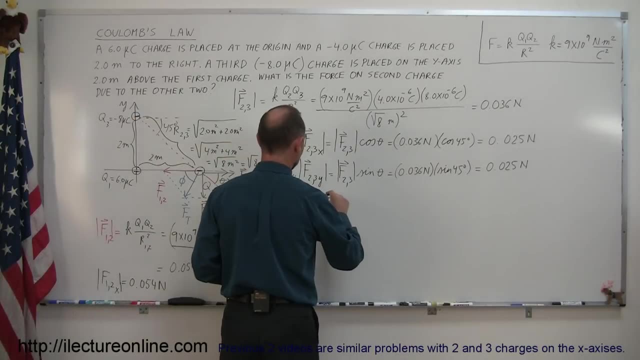 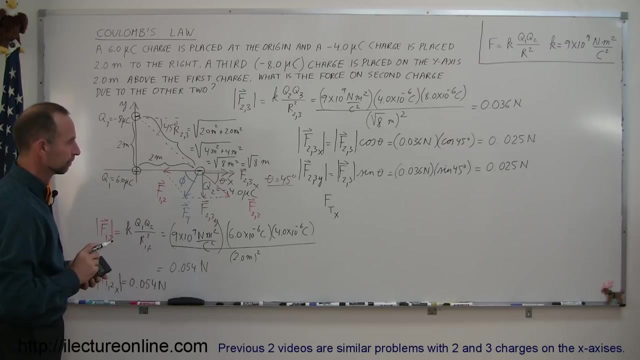 And we have the x and y components of F2,3.. Now to find the resultant vector we need to add the x components and the y components together, So we can now say that F total in the x direction. So we're going to find the x and y components of the resultant, or total vector. 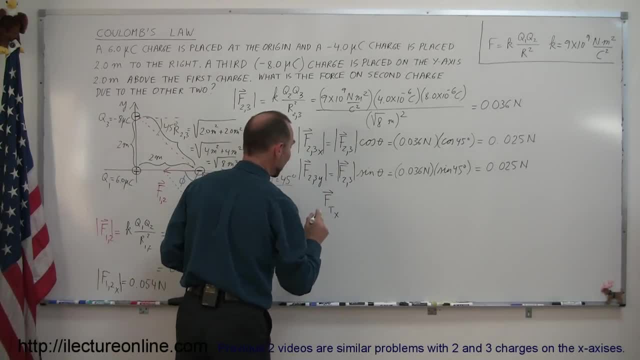 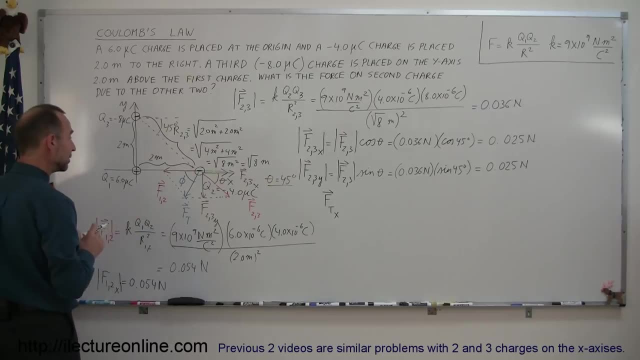 Now be careful here. Now we don't want the magnitudes anymore, Now we actually want to add the components together. And so when we add the components together we have to realize we have to deal with the directions. So I can see here that to find F total in the x direction. 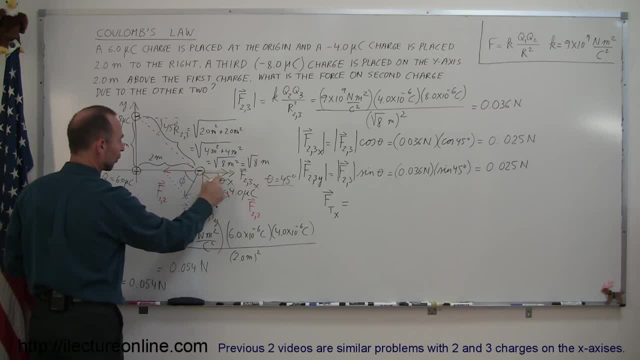 I need to add this vector with this vector together, because those are the only two components in the x direction And notice that this is in the negative direction. so F total x is going to be the minus quantity of this, minus 0.036.. 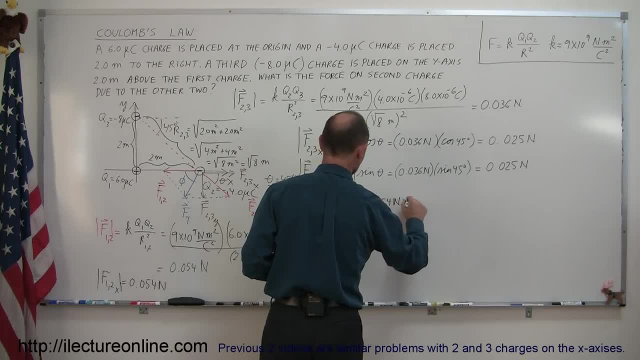 So that's going to be 0.054 newtons in the x direction. So I'm adding this component pointed to the left plus. I'm adding that component that's pointed to the right plus and that component F2,3,. we found what it was equal to. 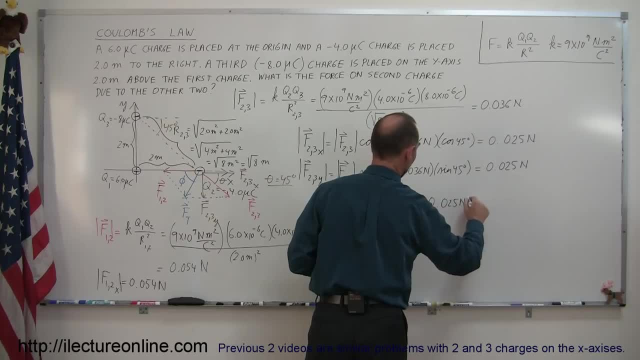 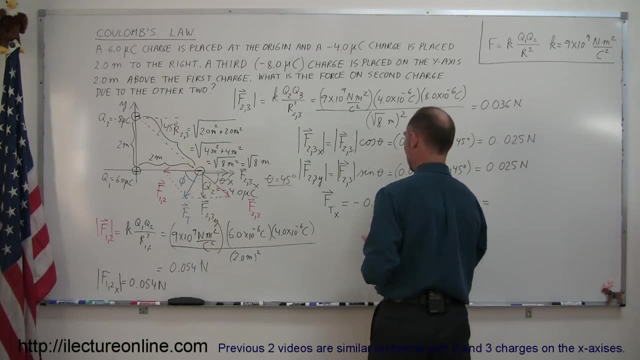 It's 0.025 newtons in the positive x direction. Okay, so when we add those two together, I can say that the x component of the total force is equal to minus 0.025 newtons in the positive x direction. 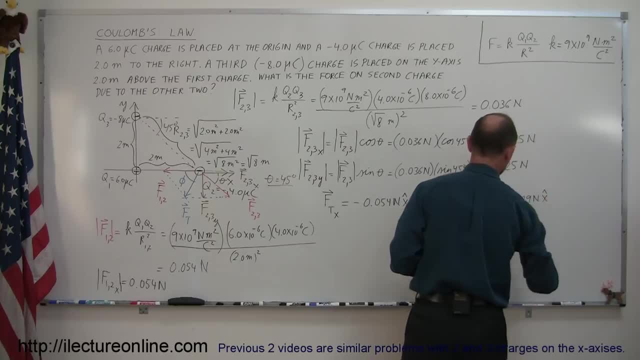 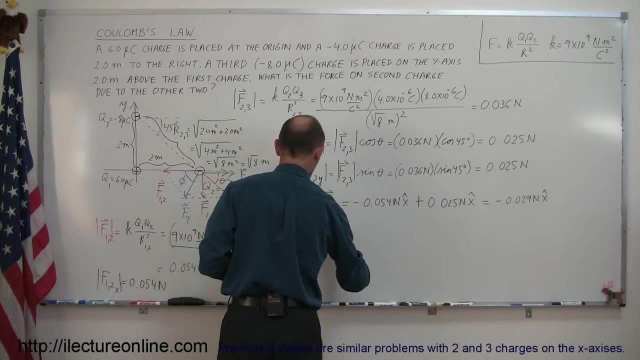 So that's going to be minus 0.025 newtons in the x direction. Okay, now we do the same for the y component. So we have the total force in the y direction, which is equal to. now notice there's no y component on our first force. 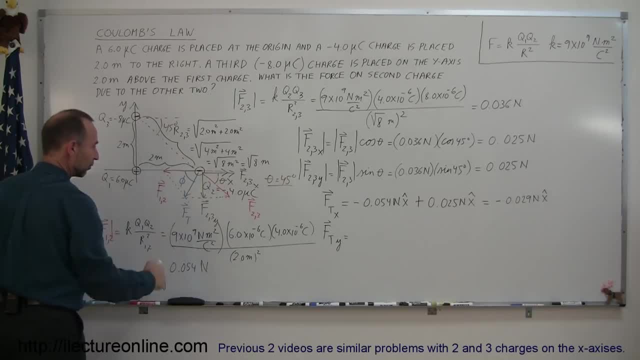 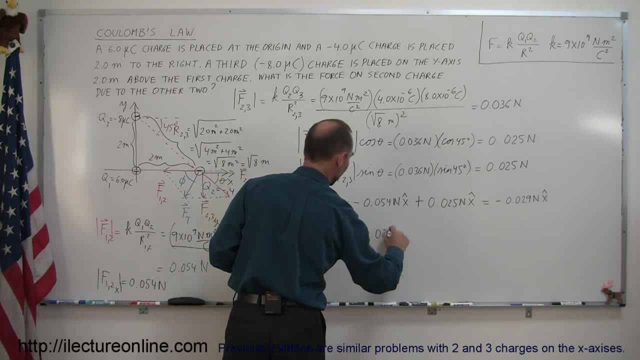 and there's one y component on the second force. It's pointing downward, so we know that's going to be negative quantity. Here it is F2,3 in the y direction, so it's a minus 0.025 newtons in the y direction. 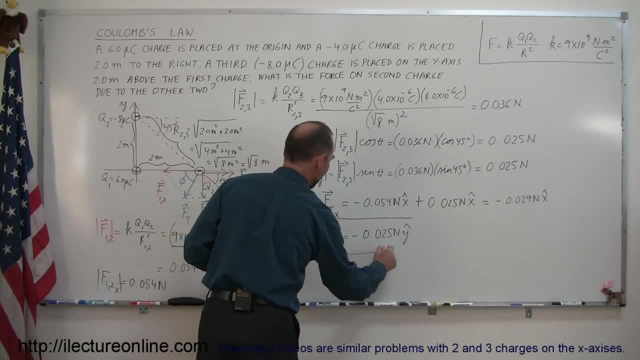 nothing else to add. So now we know that here is the magnitude of the y component, here is the magnitude of the x component. So we can now write the answer as F total, which is equal to the sum of the x and the y components. 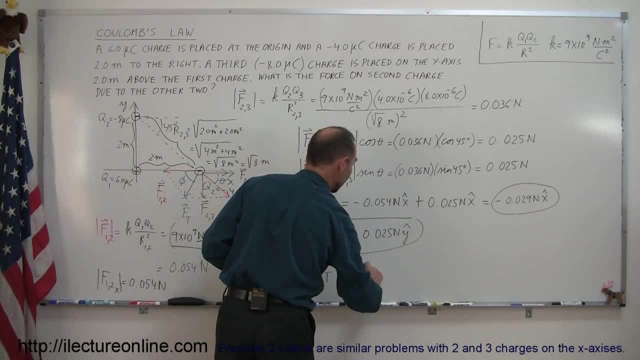 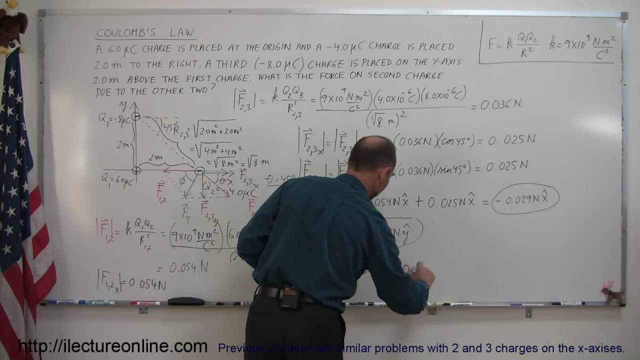 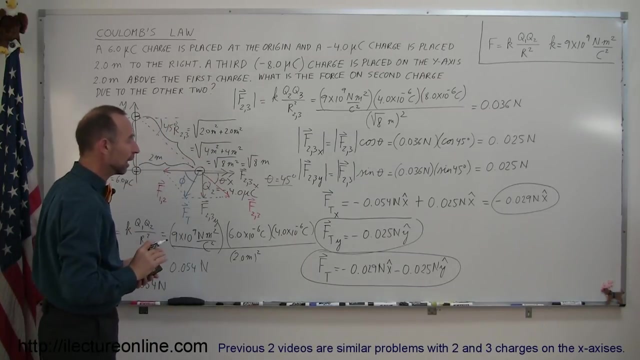 So we have the x component right here, which is minus 0.029 newtons in the x direction, minus 0.025 newtons. And here is the force, the total force on Q2 due to the presence of the other two charges. 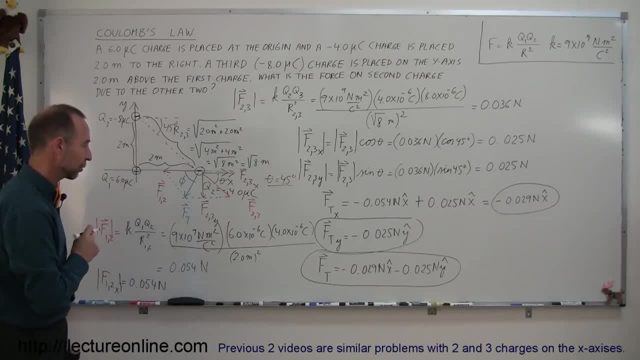 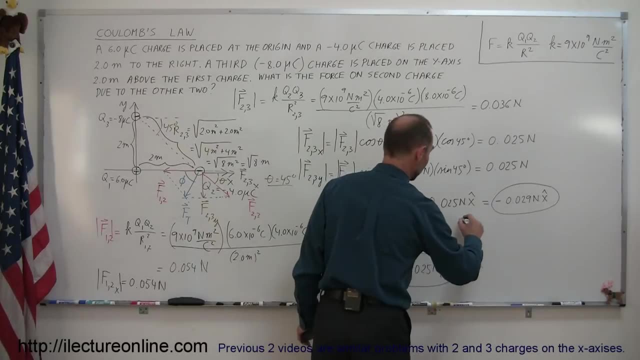 Now, that's the answer in the vector form, in the vector quantity. But what if I simply want to find the magnitude of that force? Well, to find the magnitude of the force, you use Pythagorean theorem. You can say that F total the magnitude of that. 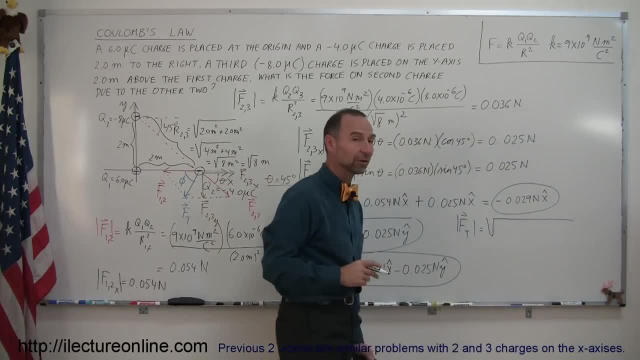 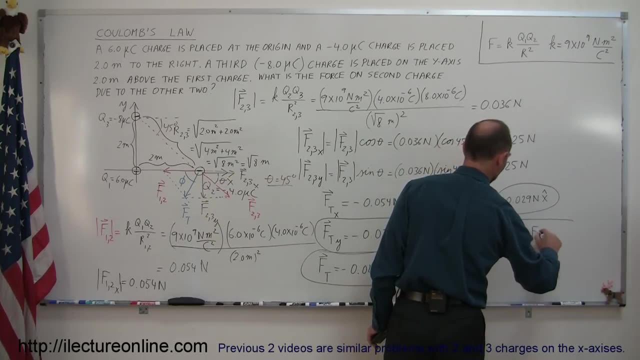 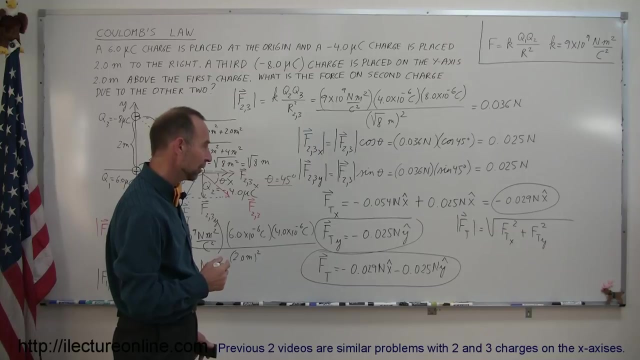 is simply equal to the square root of the sum of the squares of the individual components. So that would be equal to the F total in the x direction squared plus F total in the y direction squared. So we simply take the square, both components. 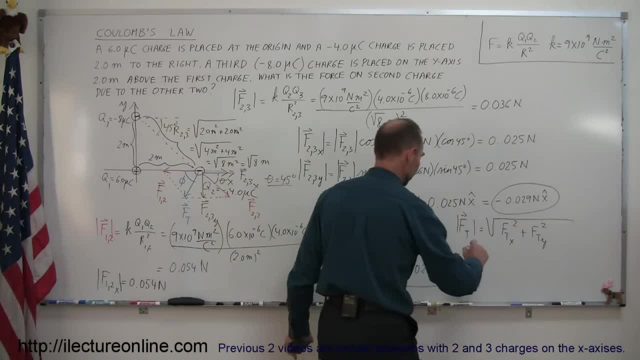 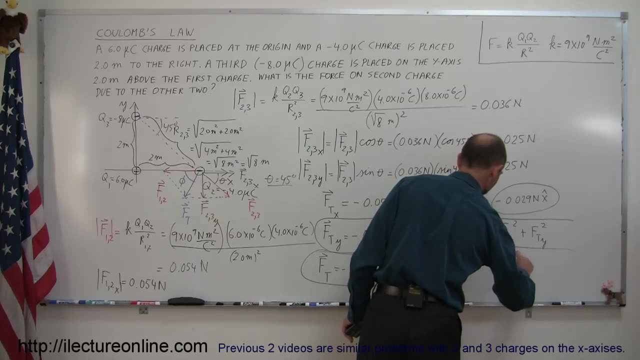 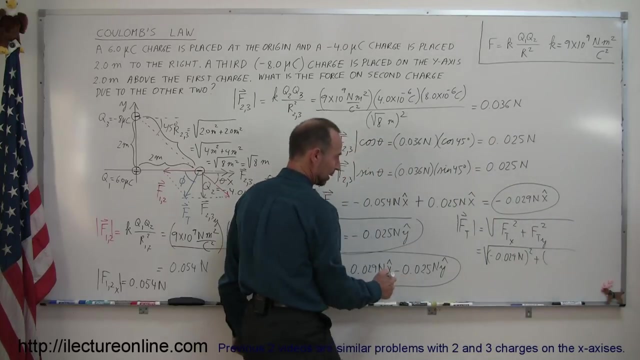 we sum them together. take the square root and that gives us the total magnitude. So this would be equal to the square root of the x component, which is minus 0.029 newtons squared plus. and then we take the y component, right here. 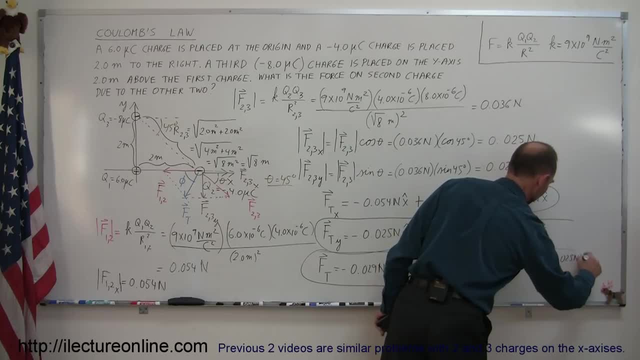 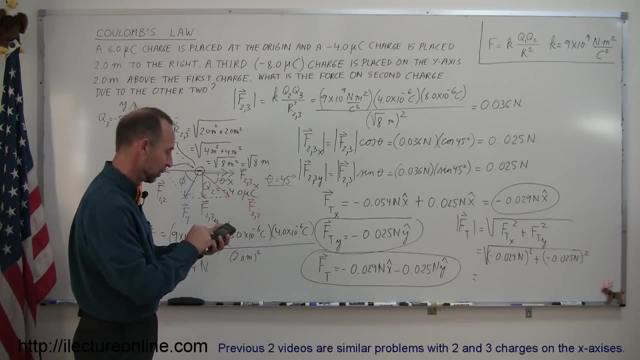 which is minus 0.025 newtons, and we also square that And what do we get when we calculate that? So we get 0.029 squared at plus 0.025 and square that. add them together, take the square root. 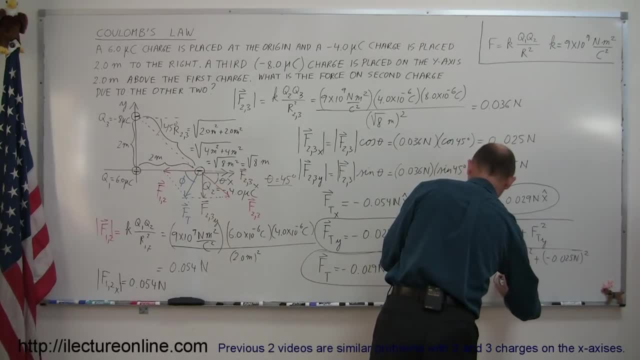 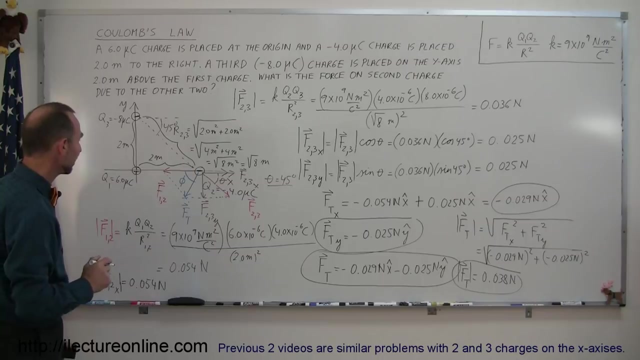 and we get that's equal to 0.038 newtons. So that is the magnitude of the resultant or total force. And then finally- and I'm running out of board space, but I think I can squeeze it on the side there- 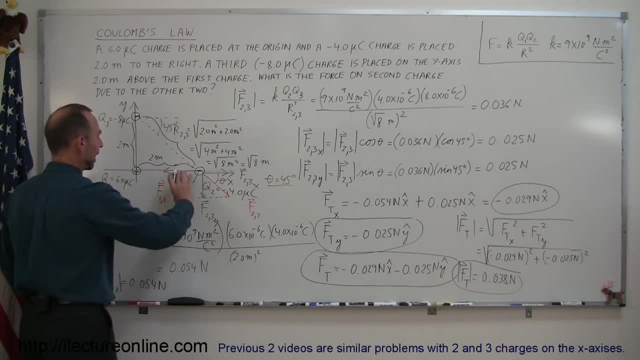 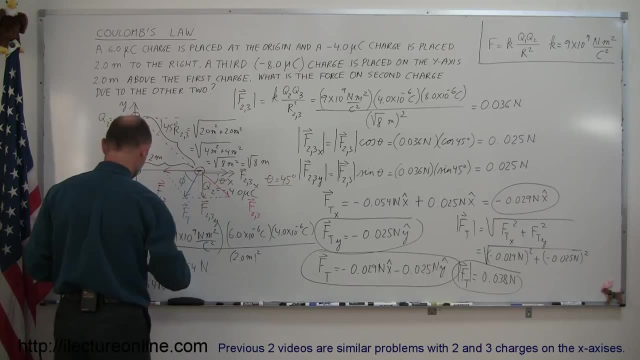 and I would also like to know what this angle is right here. So this angle is made up from the x and y components of the total force. So here we have the x component, and maybe I shouldn't use blue. Let me try this color right here. 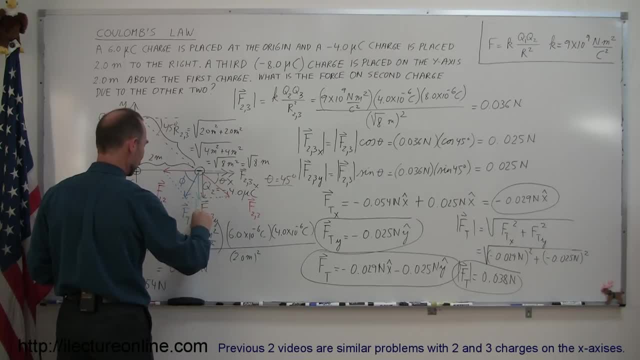 So here we go. There is the F total in the y direction and here is the F total in the y direction And here is the F total in the x direction. So those are the two components of the final resultant, the final total vector, the force on charge 2.. 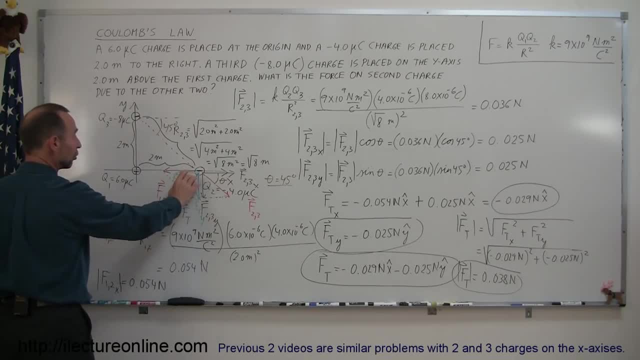 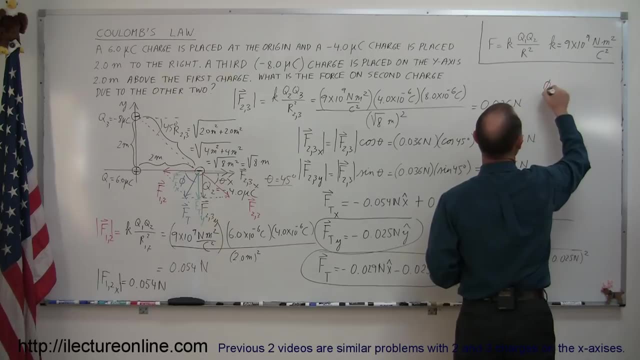 How do we find that angle? Well, we can find that by taking the r tangent. This can be like the opposite to the angle, This can be the adjacent to the angle. So we can see then that the angle phi is equal to the r tangent of the opposite side. 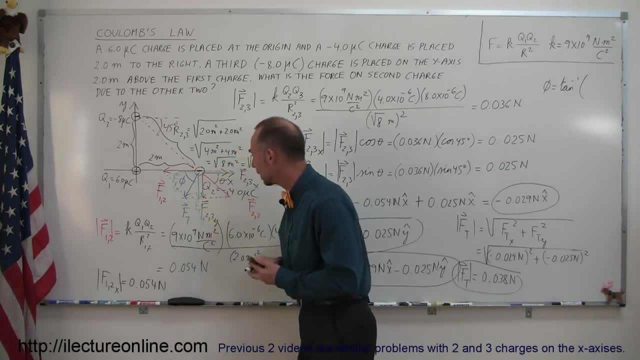 Now the opposite side to the angle would be this component. When we move it over here, that would be F total in the y direction, or at least the magnitude of that, and divided by the adjacent component, So that would be F total of the x direction. 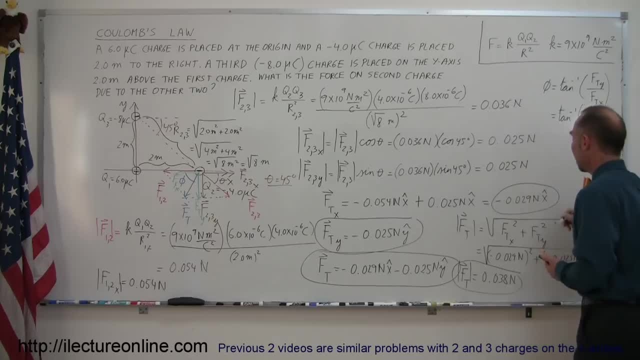 So this is equal to the r tangent of F total in the y direction. That's this one right here, Of course, we only care about the magnitudes, That's 0.025 Newtons divided by the F total in the y direction. 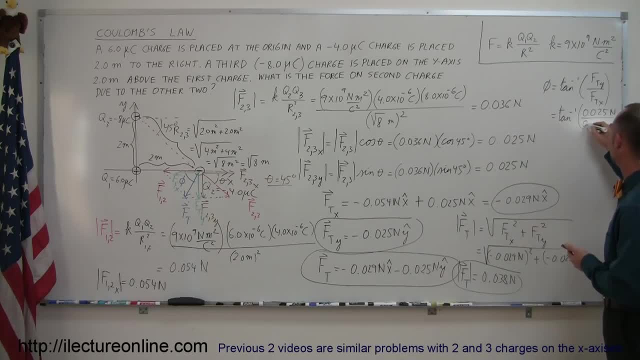 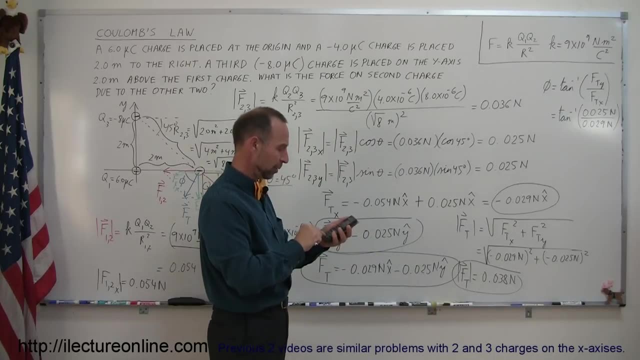 X direction. that's this quantity. right here Again, we only care about the magnitude 0.029 Newtons, like so. And when we plug that into our calculator, what do we get? So 0.025 divided by 0.029.. 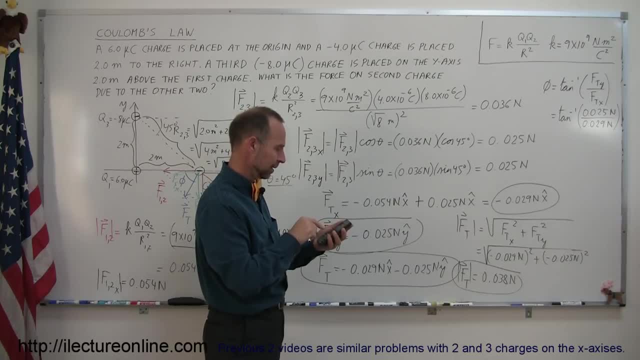 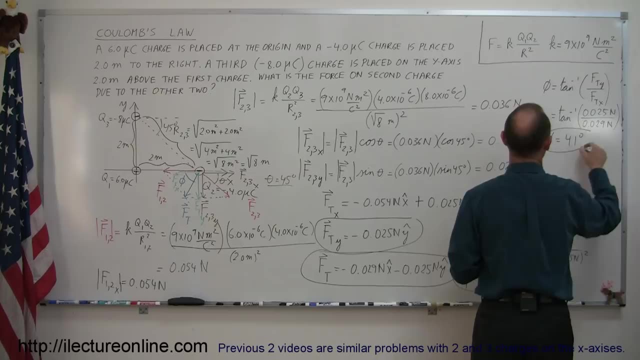 And then we take the r tangent of that And we get 40, about 41 degrees. So it's equal to 41 degrees phi. There we go. So there's two ways of looking at this answer. We found the resultant. 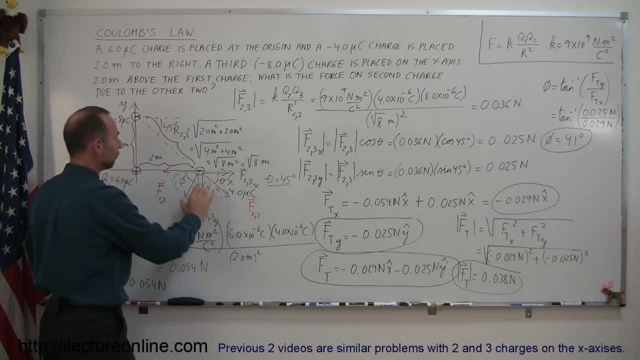 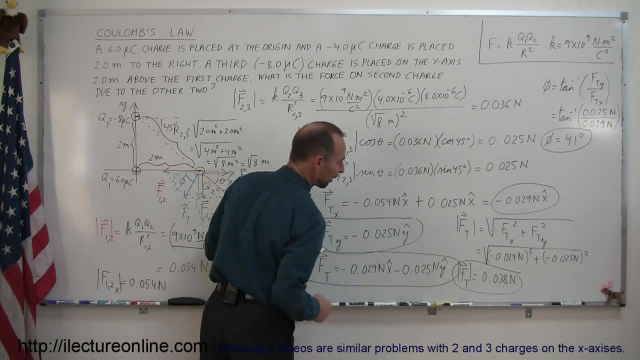 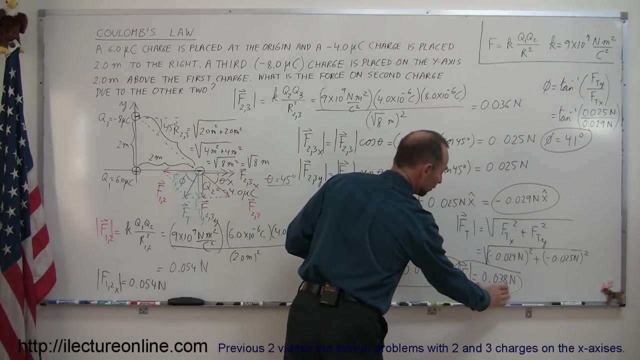 This is the resultant vector. The total force on Q2 is equal to negative 0.029 Newtons in the x direction, minus 0.025 Newtons in the y direction. So we wrote it as the sum of its components, Or you can think of it as the magnitude. 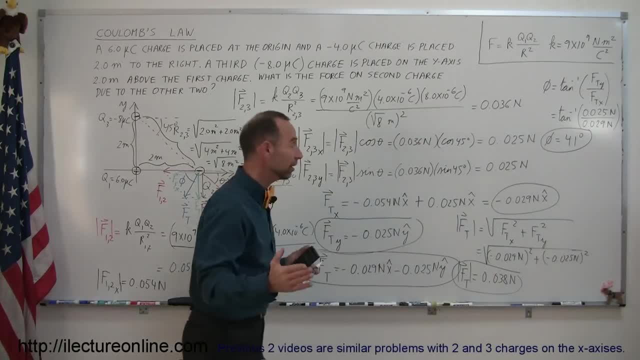 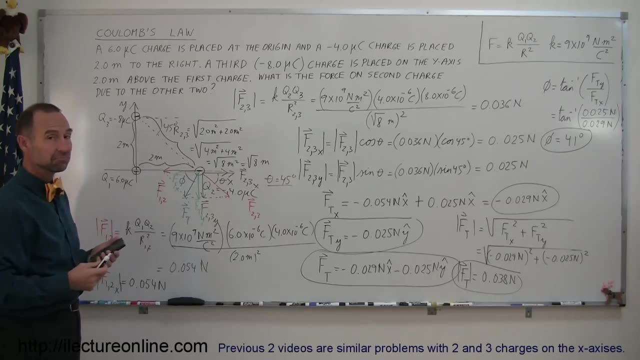 This is the magnitude of the force And that's the direction of the force, relative, in this case, to the negative x axis. And that is how you do one of these problems. They're very lengthy, But just to quickly summarize how you go through this problem: 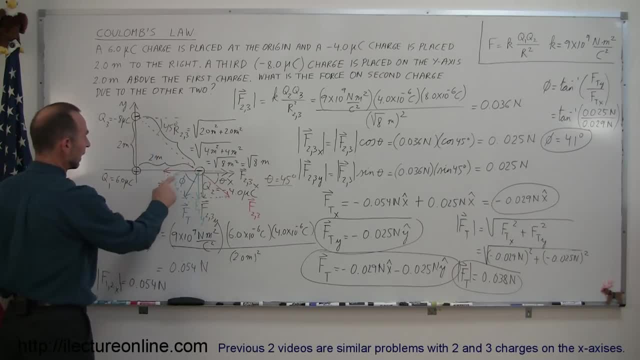 you first make a diagram of where the charges are, Then you draw the forces on the charge in question And you want to find the force on this charge relative to the presence of the other two. So you draw a vector representation, using the arrows, of what those forces are.